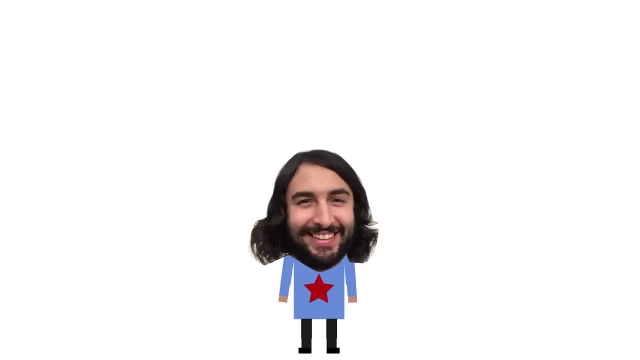 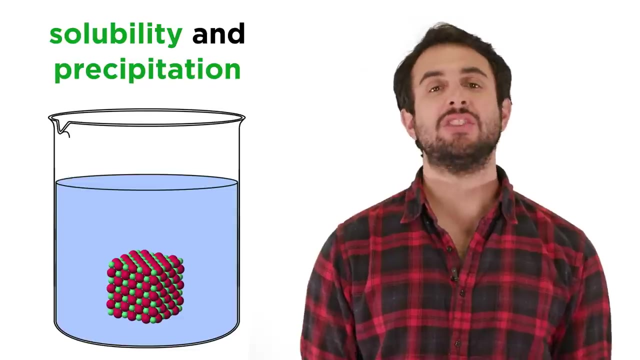 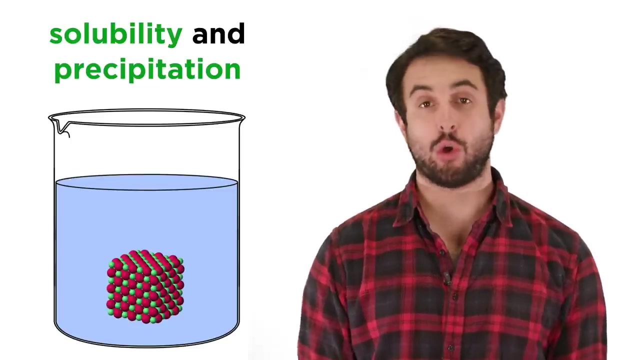 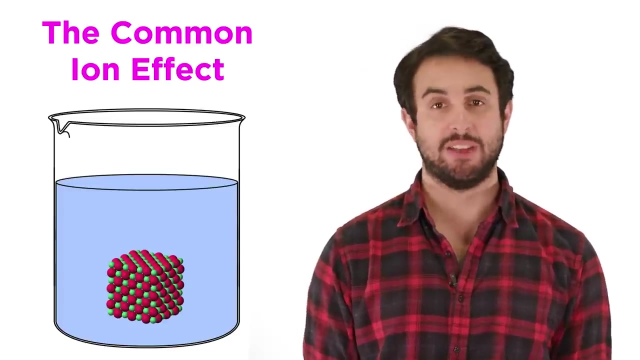 It's Professor Dave. let's learn about the common ion effect. As we continue to learn about solubility and precipitates, we are beginning to understand ways that we can predict or even control precipitation. One such approach we must understand involves something called the common ion effect. so 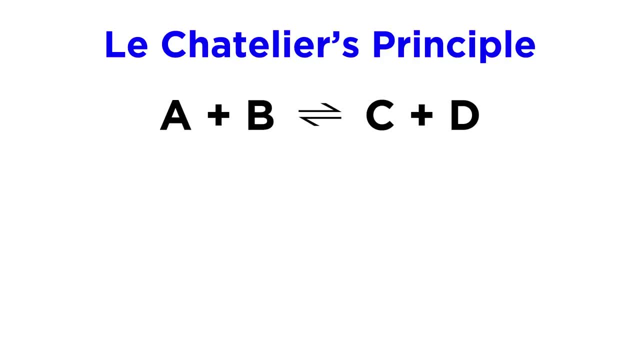 let's learn precisely what this means. The common ion effect is an application of Le Chatelier's principle, which we learned all about in an earlier tutorial, so if you need to review, check that out now. Otherwise, we know that under this principle, which describes the behavior of equilibria, 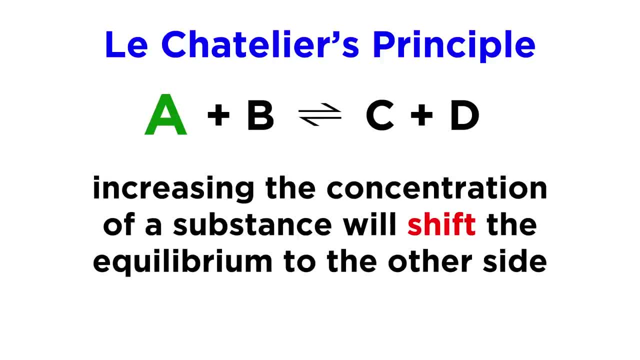 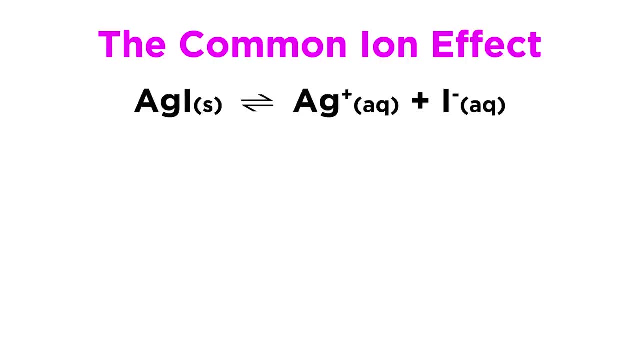 if we were to add an additional amount of one of the components in an equilibrium, the equilibrium would shift towards the other side, using up some of that additional component and creating more of the substances on the other side. Let's now look at an equilibrium between, say, silver iodide and the aqueous silver. 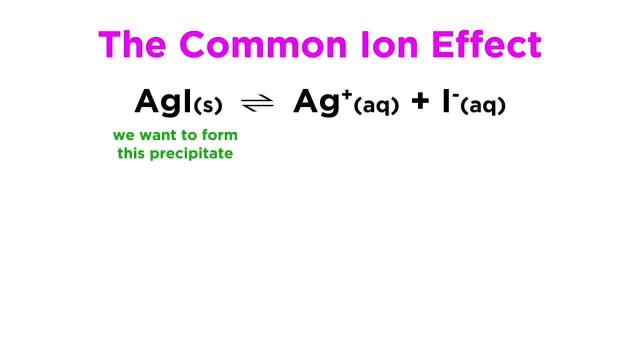 and iodide ions. If we are interested in forming a silver iodide precipitate, one way we can do this is to add some potassium iodide. Potassium iodide shares a common ion with silver iodide, that being the iodide ion. 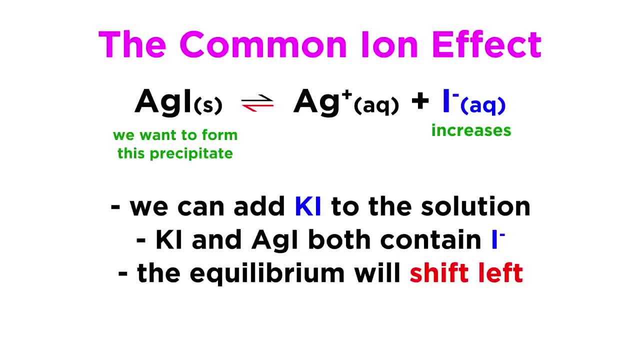 If there is more iodide ion in solution, that will affect the equilibrium. Potassium iodide shares a common ion with silver iodide, that being the iodide ion. If there is more iodide ion in solution, that will affect the equilibrium and it will. 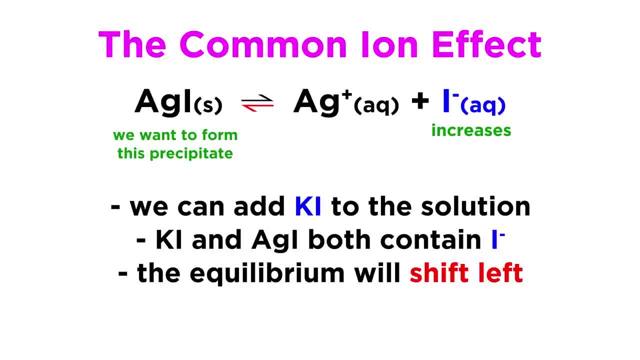 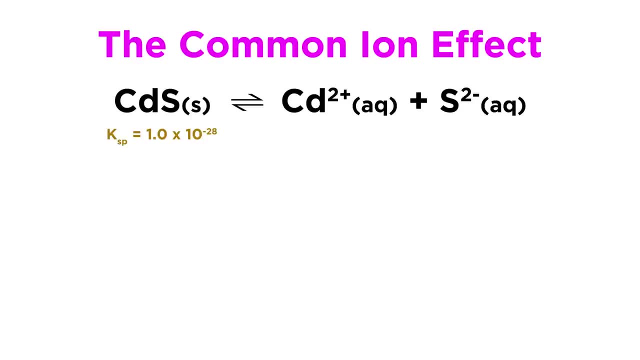 shift left to use up the excess iodide ions. If the equilibrium shifts left, that means more silver iodide precipitate will form. so this is a method of promoting precipitation. Let's look at this more quantitatively. Cadmium sulfide has a Ksp value of 1 times 10 to the negative 28.. 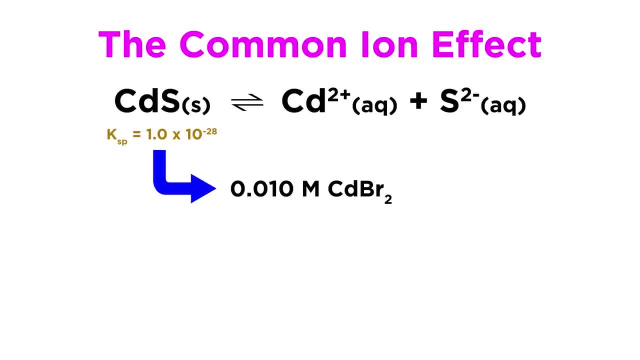 If we place some cadmium sulfide in a 0.01 molar cadmium bromide solution, it will be 0.01.. If we place some cadmium sulfide in a 0.01 molar cadmium bromide solution, what will? 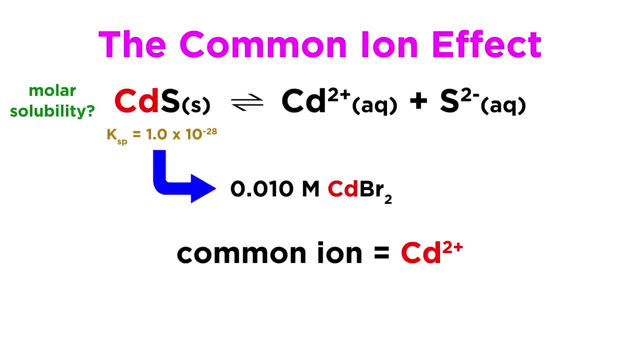 be the molar solubility of the cadmium sulfide. So first we must recognize that the common ion in this situation is cadmium, as it is present in both compounds. Let's then set up an icebox for the cadmium sulfide equilibrium.